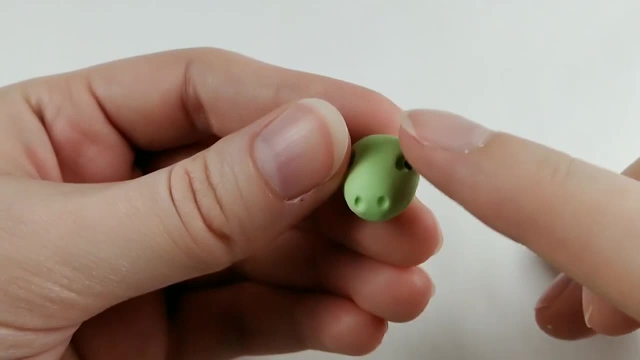 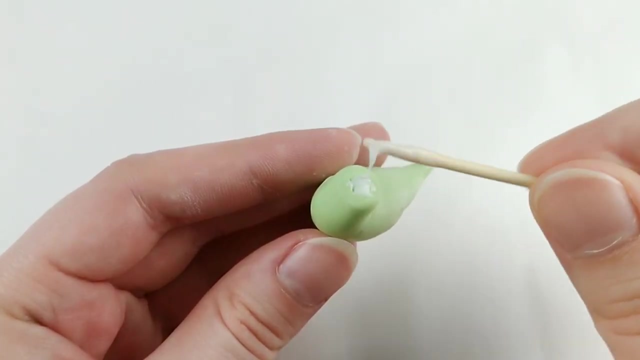 but now it kinda looks like it has cheeks. so we'll call it a happy accident and move on to adding little black balls for the eyes. We can now attach the head to the body using a bit of liquid Sculpey, Press it in place and blend into the neck with a ball-pointed or. 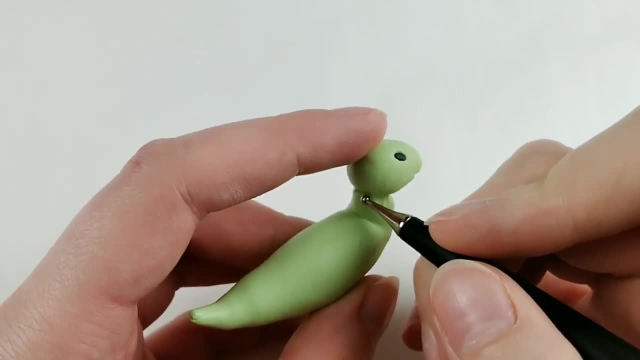 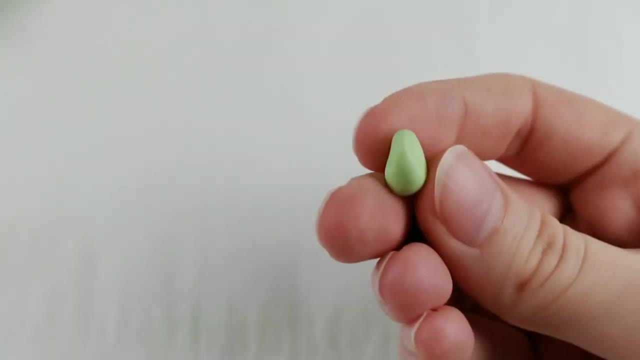 angled sculpting tool. The face got kinda squished, so next time I'll add the face details after attaching the head. For the legs I'm squishing a ball into a teardrop and flattening the edge to make attaching easier. 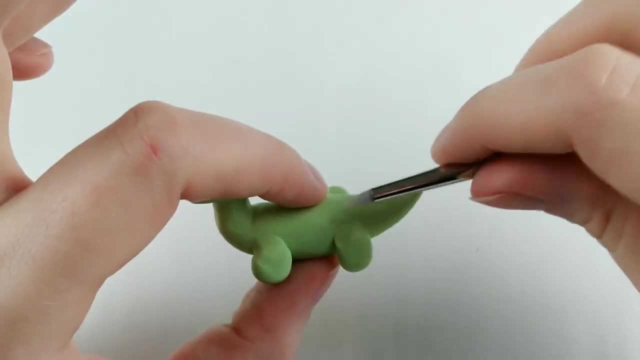 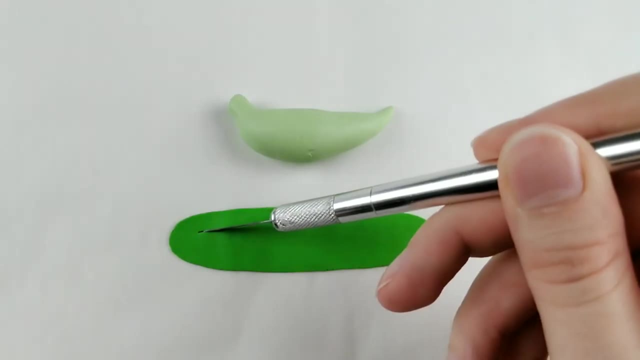 Once the legs are on, you can blend with either a silicone tool or your finger And when you're done, it should look something like this: Onto the belly, I'm choosing a darker green and flattening it out before cutting into shape. 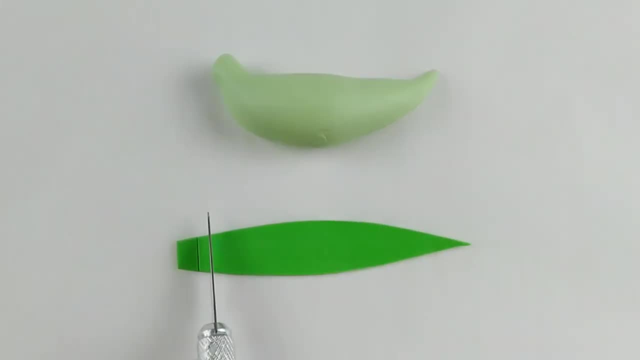 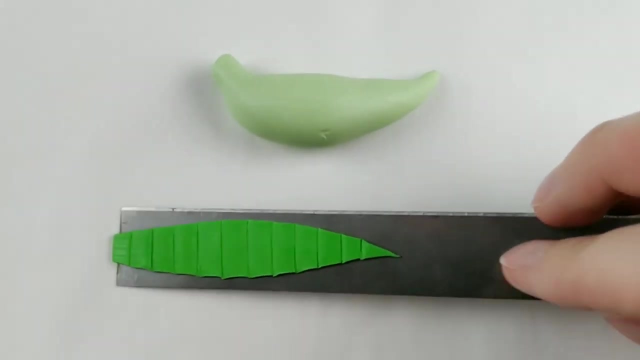 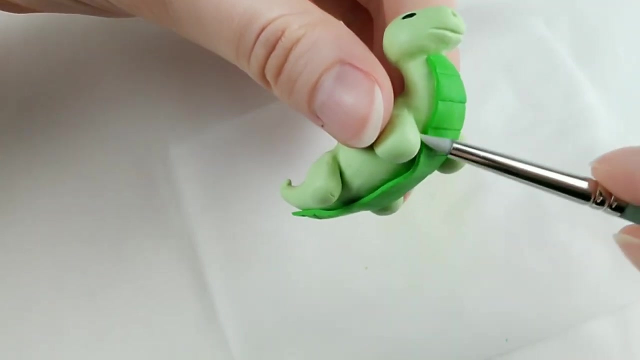 You can use your dragon as a cutting guide to better estimate the length you need. Once cut, scales can be added with a blade or flat edge tool. Then after a little liquid Sculpey, it's added onto the belly. I used a flat edge tool to press everything into place. 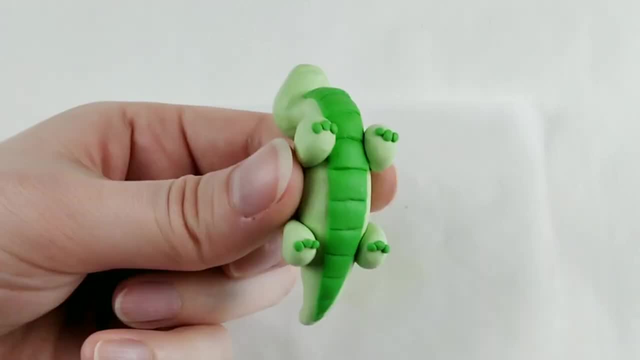 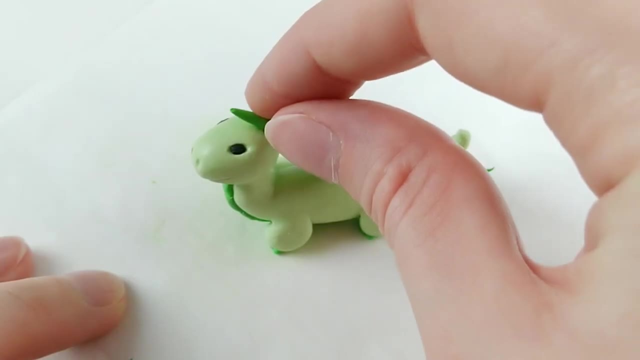 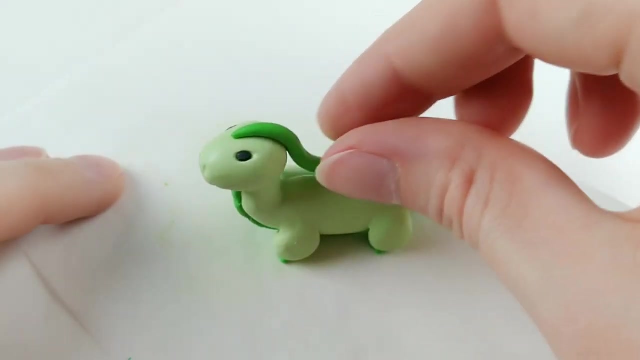 And we can't forget about the little toes For the scales going down the back. I'm rolling out another ball of dark green clay, but this time into a log the same length as the dragon. Add some liquid Sculpey, then time to give your dragon a really long side bang, Or I guess you could continue to. 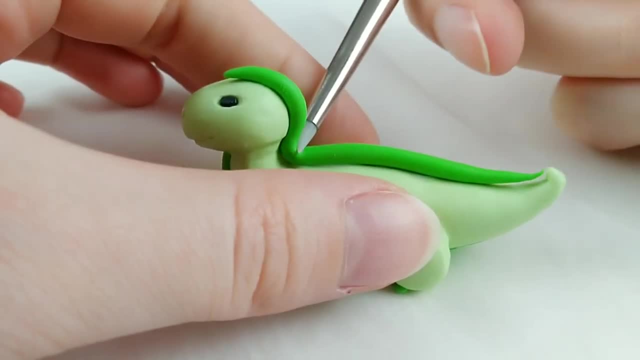 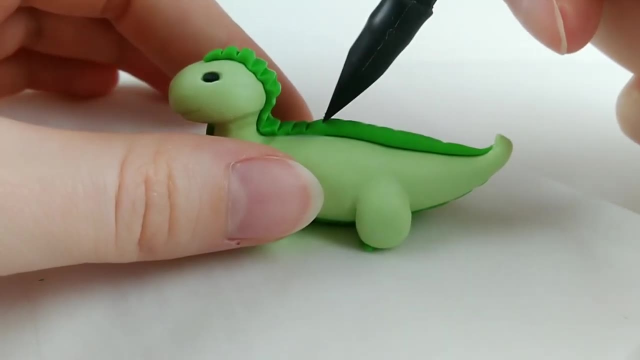 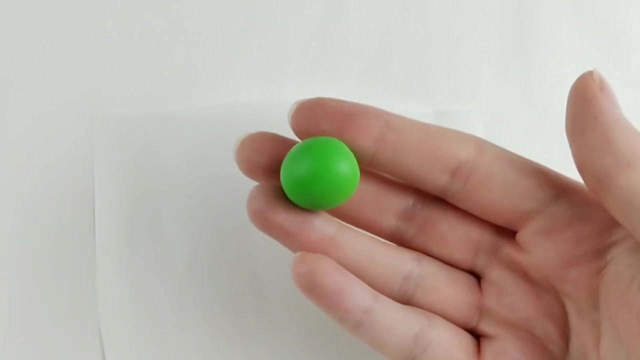 attach it down the rest of the body until it reaches the tip of the tail. From there we're going to recreate the look of individual scales by using a flat edge tool to indent all the way down the length of the body. This is an easier way to add detail to your dragon. but since I'm making 3 dragons today, 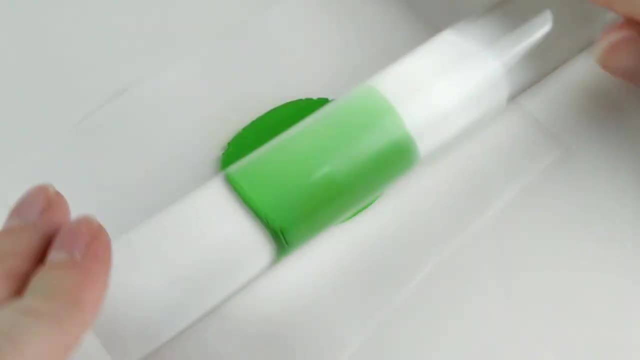 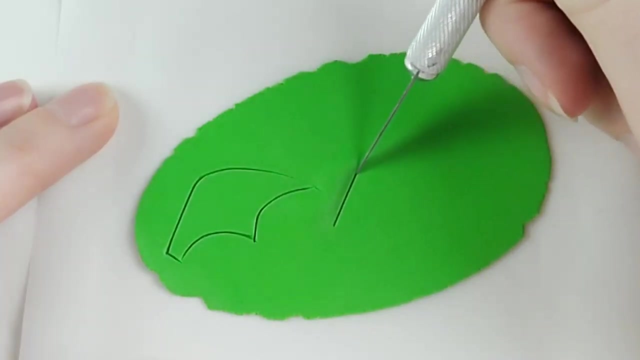 I figure I'll show you 3 different ways to make the scales and the wings, Using the same dark green as before. roll out a thin sheet and cut into your wing shape. I drew mine facing the same way, since it seemed like it would be easier to tell if. 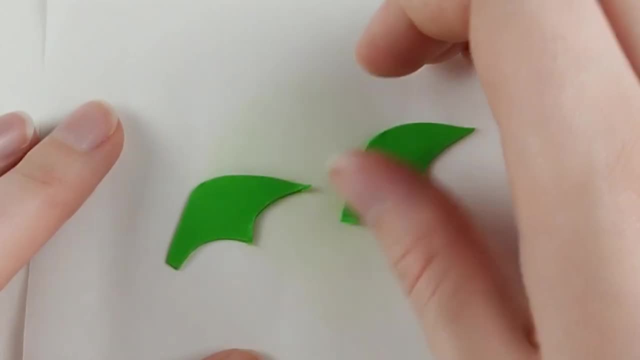 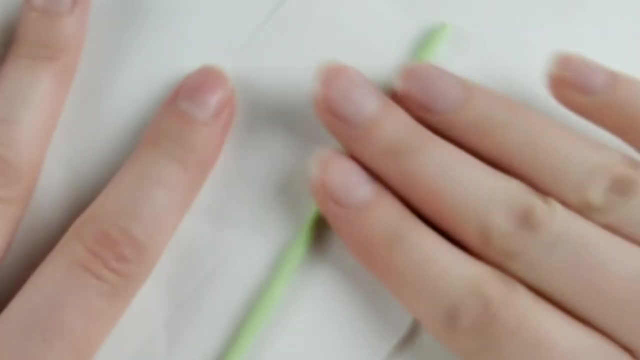 the wings matched each other, Then I just flipped one around to face the correct way. Technically this didn't matter, since I'll be making these wings the same on either side. To do this, I first add light green details for the wing support. 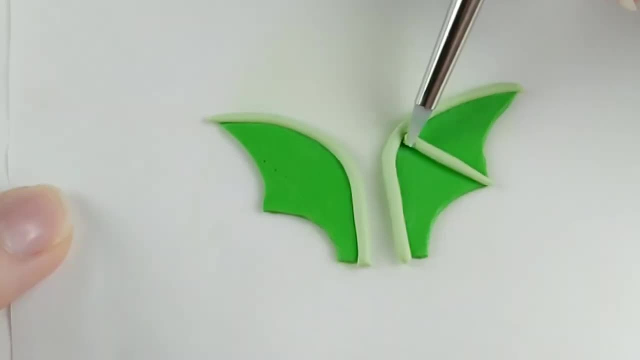 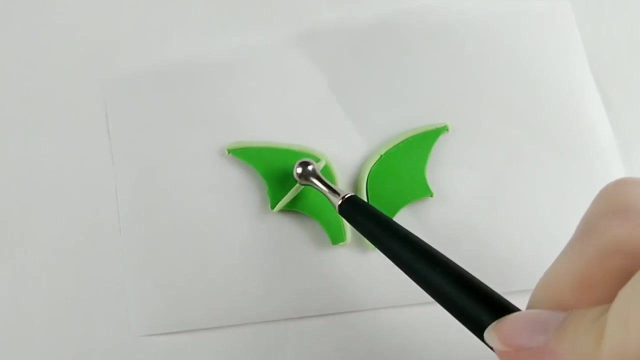 and one down the middle to create two sections of the wing. Once one side is done, I lay another sheet of parchment paper on top and press it down. When I flip it over and peel the other layer of parchment away, the wings will stick to. 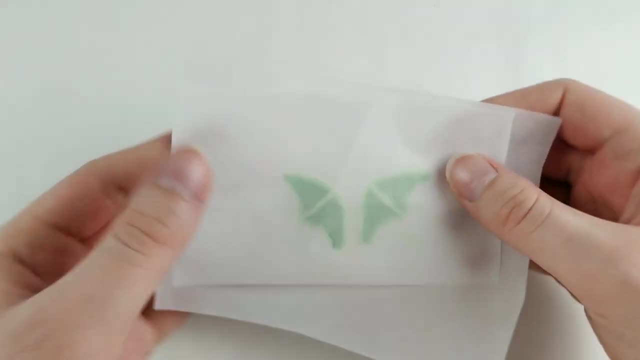 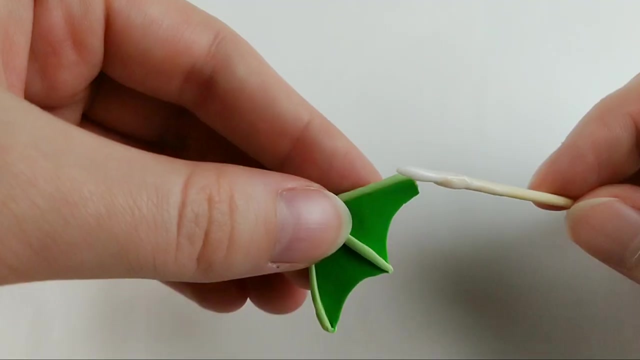 the bottom sheet and I can now add detail to this side. Now, to make these easier to add to the dragon, let's give these a little pre-bake first, And all that's left to do is to add some lucid sculpey to the end and push it into the body above the front leg. Same on the other side. 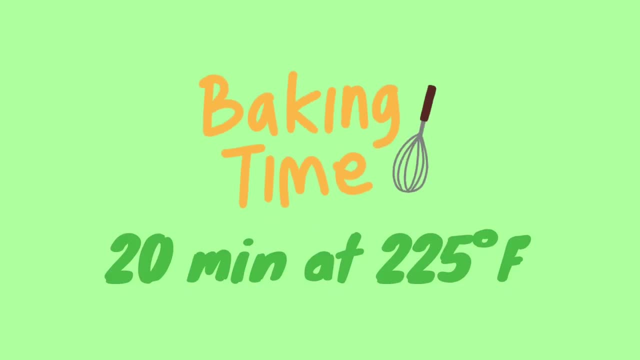 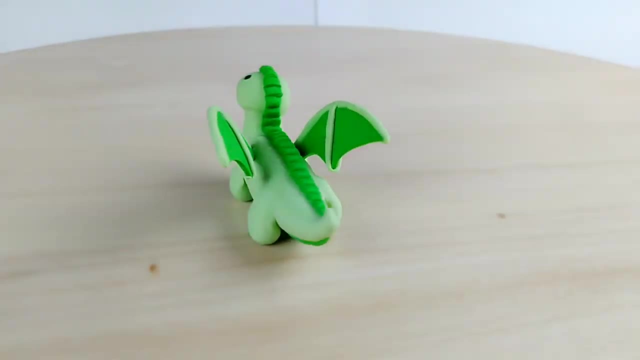 and this dragon is ready for its final trip to the oven, Freshly baked, and our first dragon is done. The smushed face looks a little derpy, but it's not bad for a first attempt. Onto the next one. Grabbing some blue clay, I'm rolling it out the same way as before. 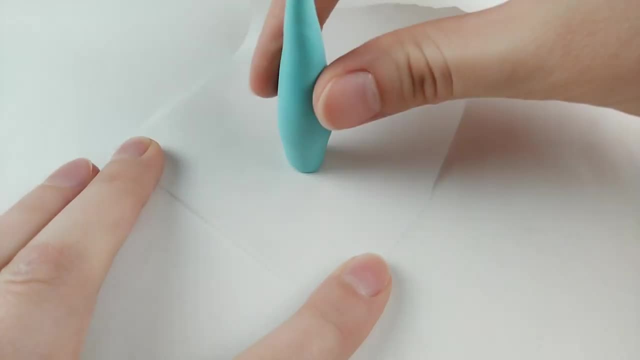 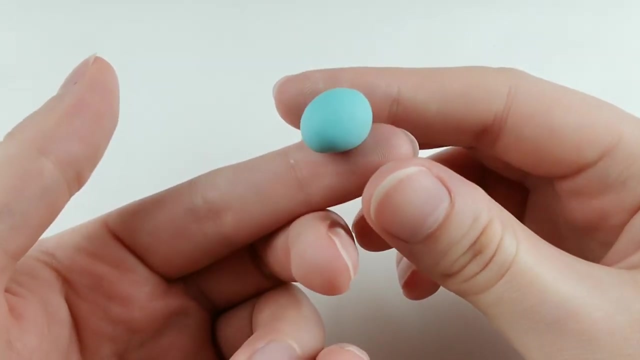 but I'm leaving it a little thicker, since I want this to be a cute chubby dragon. After bending the neck and the tail up, I'm taking a small ball of clay for the head and leaving it nice and round, with no extra shaping Intents for the eyes and 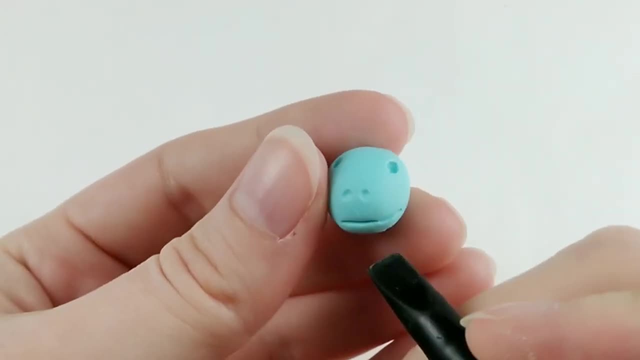 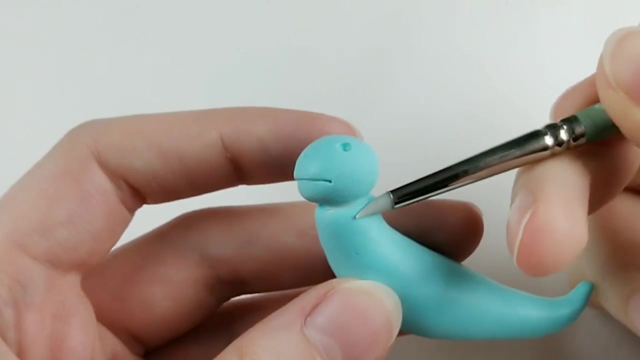 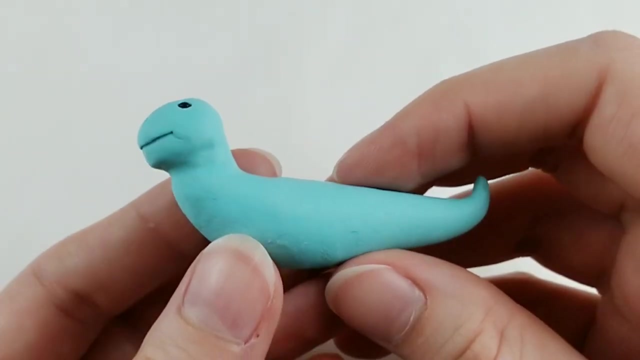 nostrils and a smile accompanied with some chubby cheeks. We learned from last time to add the eyes later, so let's go ahead and attach it to the body now, Blend together with an angled silicone tool, and now seems like a great time to add the eyes. Time to give this slug some legs. 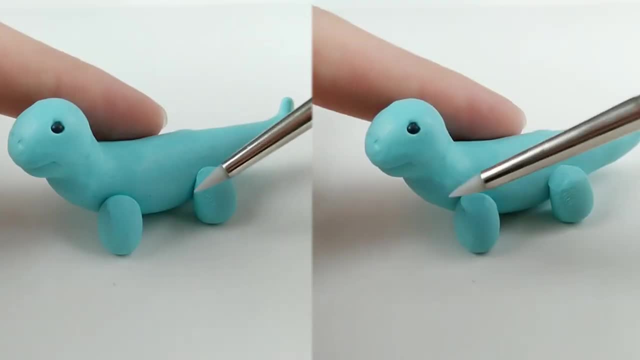 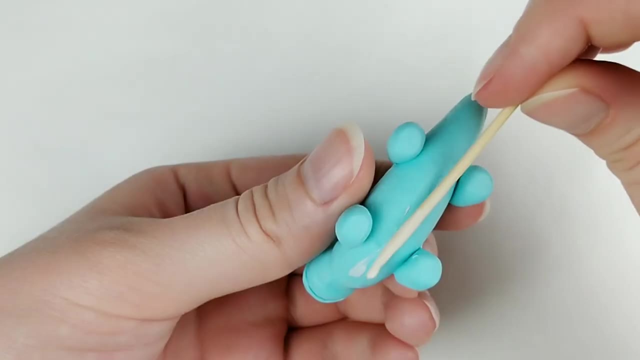 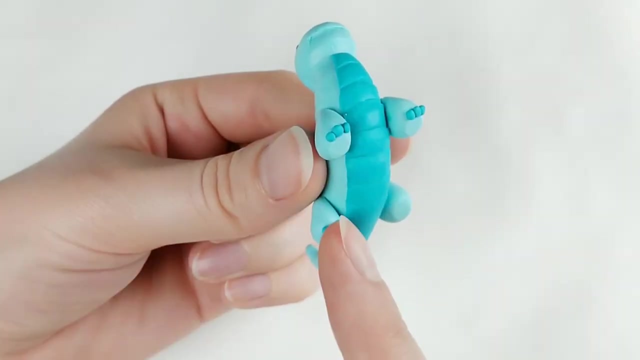 And, once attached, I'm blending them in, as well as using a q-tip dipped in acetone to both blend the legs even smoother and pick up dirt that the clay always seems to find. Another scaled belly gets added to our dragon, as well as some little toes or claws, if you can even call them that. 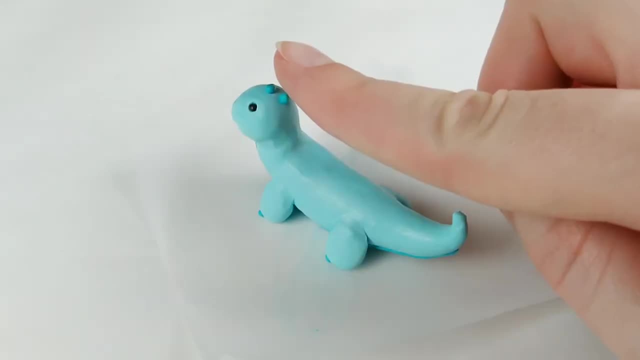 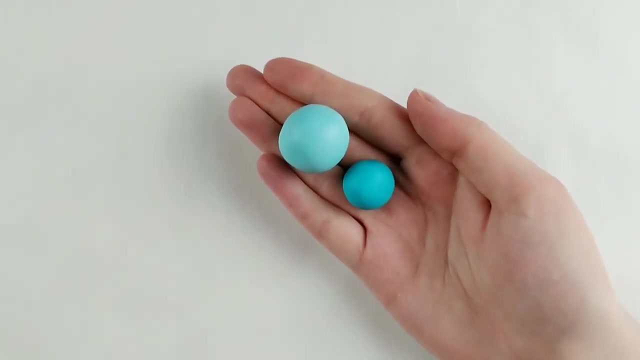 Now for this dragon's scales. I decided to play up the cute theme and choose to add rounded scales down the back, With the smaller scales on the head that get larger towards the middle of the body and then taper down at the tail. I added a dot of liquid Sculpey to each one to ensure that they'd stay in place after baking. 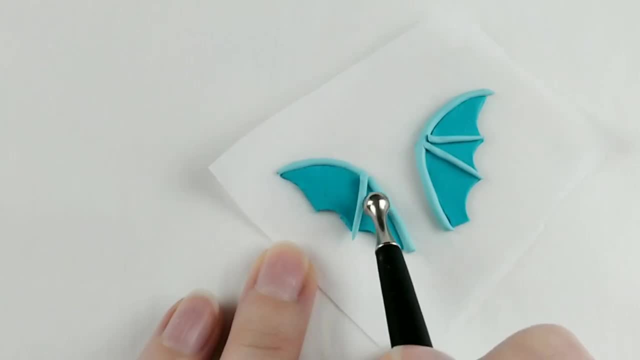 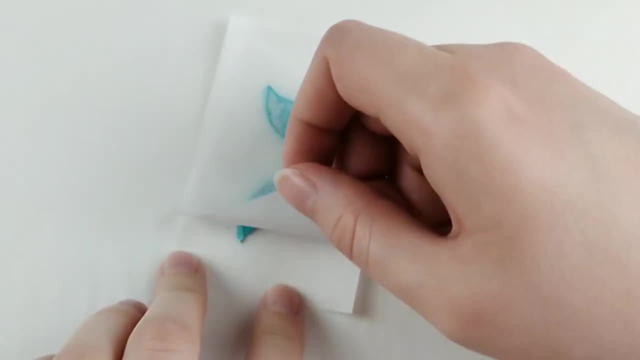 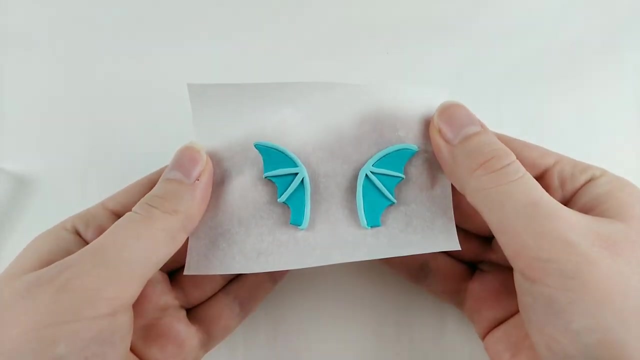 Onto the wings, where I decided to make them a bit more detailed than the first, with this one having three sections of the wing instead of two. Once again, I'm adding the light clay color for the wing arms and flipping over to repeat on the other side, And same as before. we want to pre-bake these before attaching to the body. 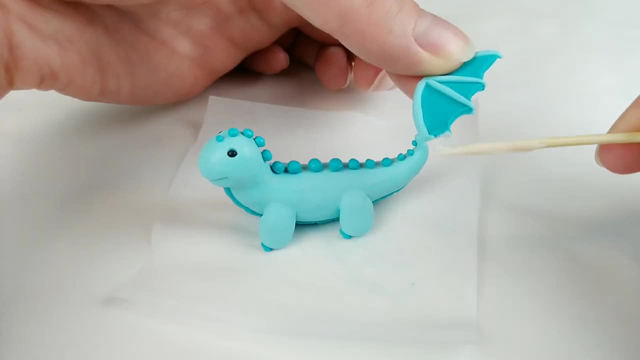 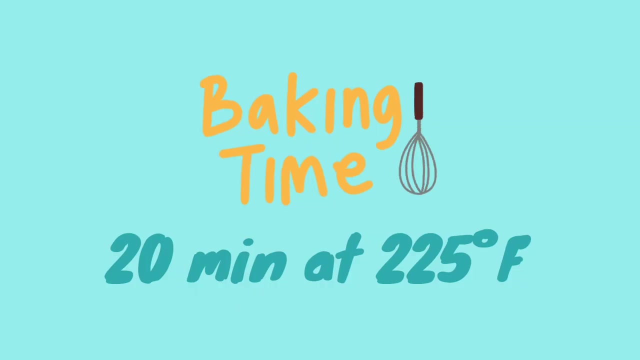 You can try and add them without pre-baking, but I guarantee you won't have a fun time. Now, with the wings in place and secured with liquid Sculpey, it takes a final trip to the oven. I think this one turned out super cute and I love the little cheeks on either side of the smile. 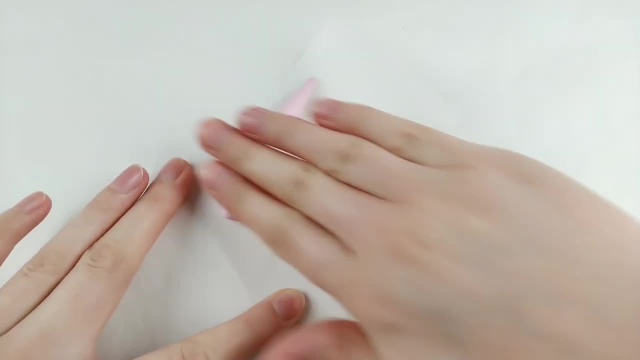 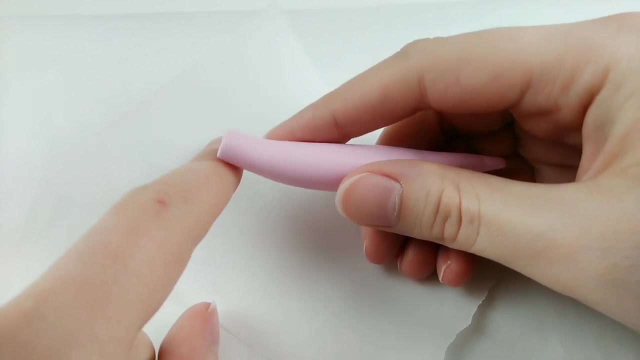 The pink dragon is last but not least and for this body, when I roll out the clay, I'm really trying to elongate the neck and tail to create a different look. The neck will be bent the same, but the tail will look much nicer if the hair stays straight and while at an angle, it will help to smell more drei-eline-like direct gems. 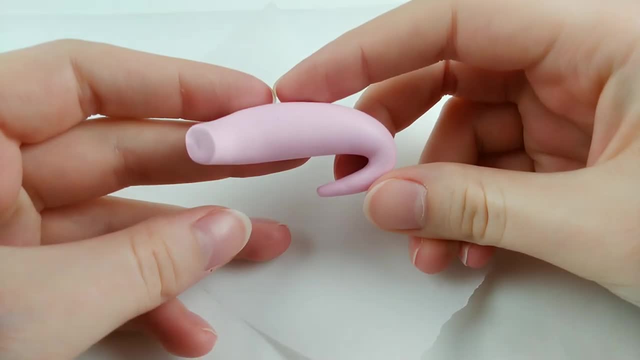 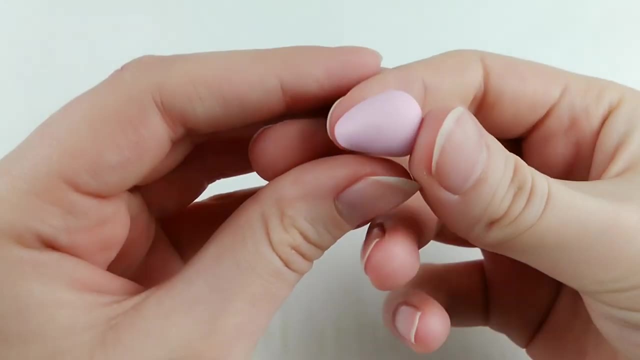 now be turned towards the front instead of flipped upwards. The head will be shaped more triangular by pinching one end of the ball to create a cone shape, And I figure there's no harm in attaching the head to the body now, since there was still a bit of squished features on the last dragon. 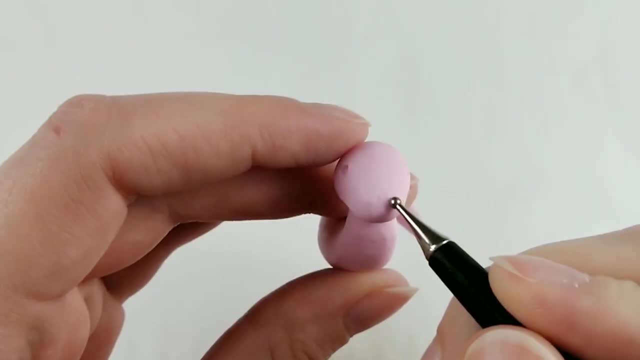 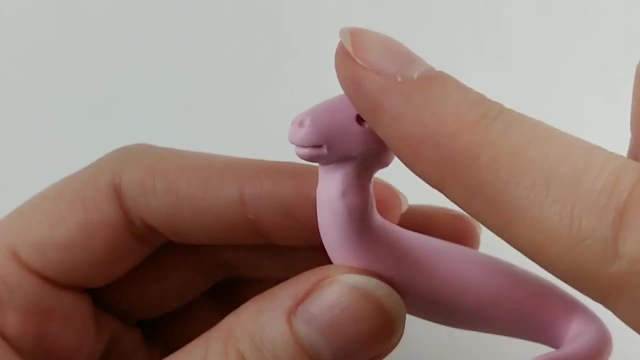 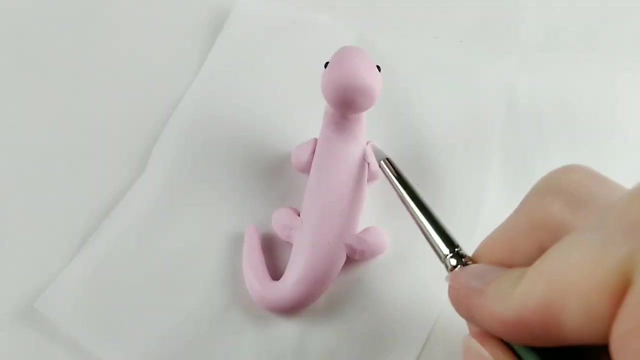 I find that every new dragon I make gets easier and takes less time than the one before. I'm considering making more mini dragons to complete this half rainbow. I already have Maybe even one with multiple heads. I can definitely see this becoming an obsession to create my own little miniature army of dragons to guard my clay treasures. 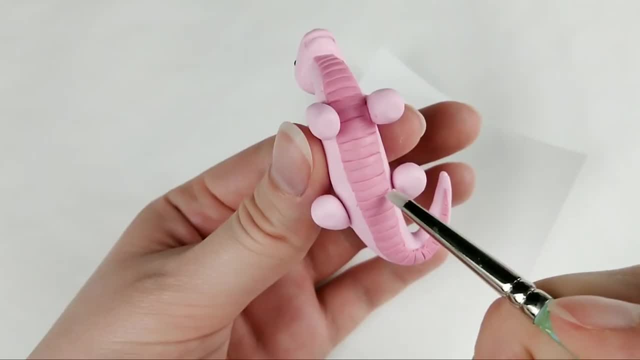 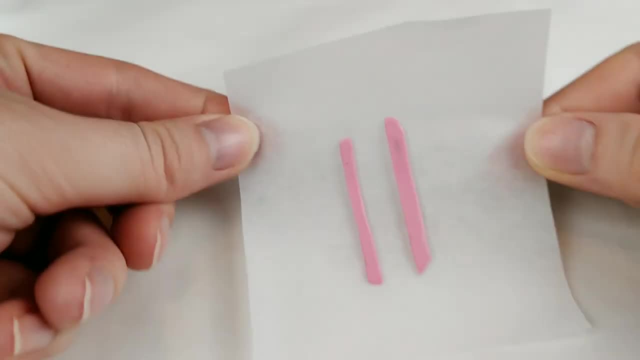 so let me know if that sounds like something you'd want to see. I'll gloss over the scaled belly and the toes, since you've already seen it twice before, but the back scales will be something new. I cut out two thin strips of dark pink. 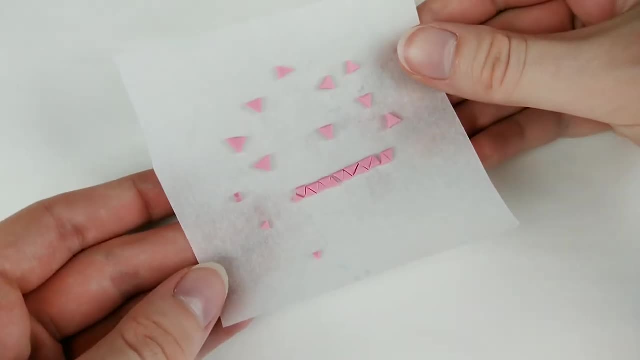 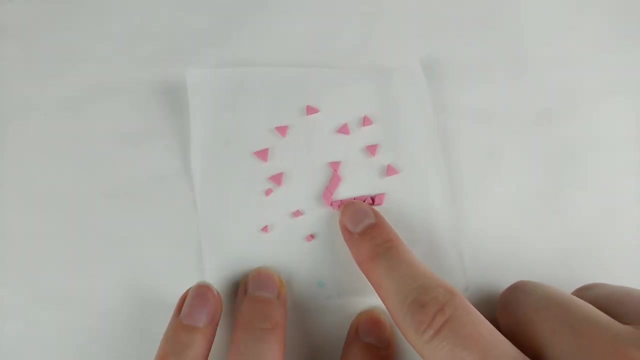 which I will then use to cut out a bunch of different sized triangles, Then to set the shape. we're going to pop these in the oven for five minutes. Once out and cooled, it's time to break them apart and sort them in ascending to descending order. When you have enough, start attaching them to the body with 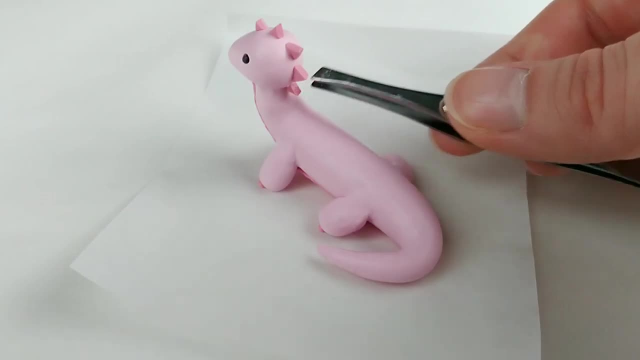 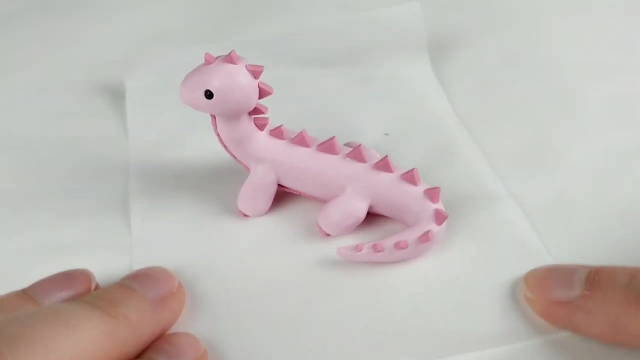 a bit of liquid sculpey. I'm using tweezers to place these, since I knew my fingers were going to be way too clumsy for the job. Now continue along the curve of the tail, finishing with your smallest piece. Time for wings. 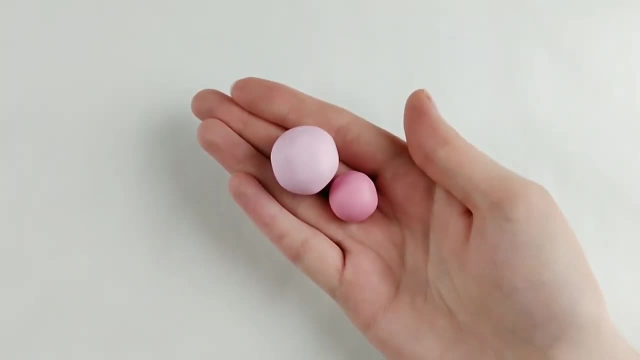 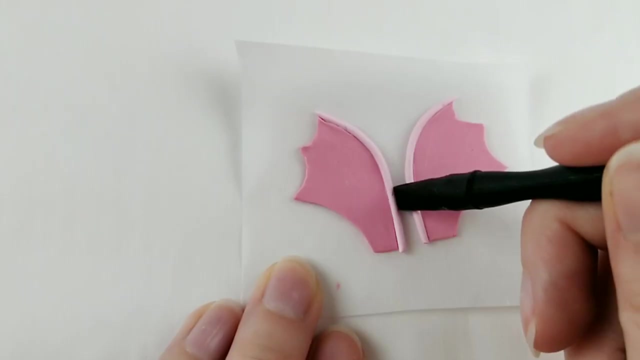 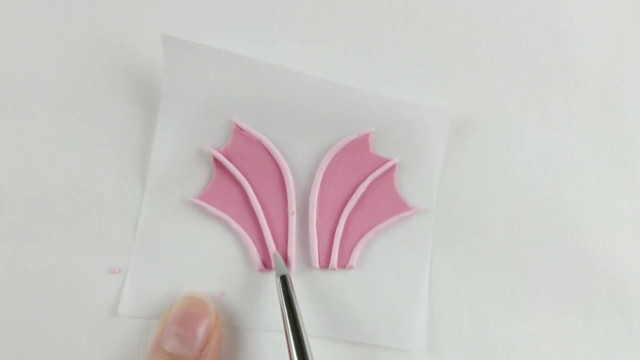 These wings are a little different. They're less triangular and more of a long curve, Reminds me of a fish fin than a wing, but I like it and it's always another design for you to try out. While I'm choosing to add detail to both sides of the wing, it would look perfectly fine on just. 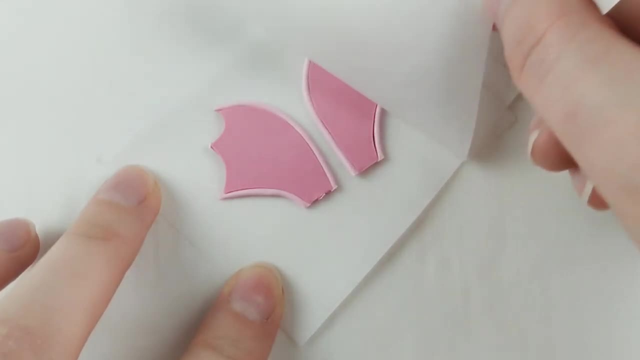 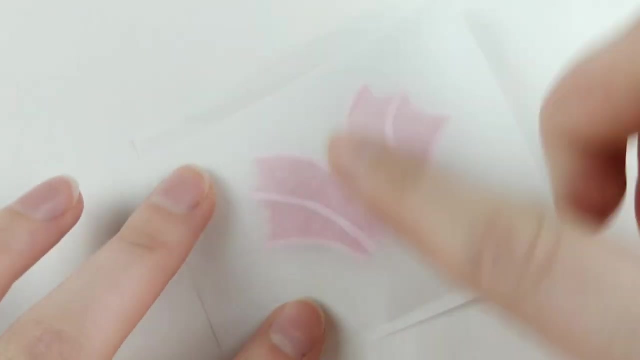 one side, especially if you attach the wings closer to the body. Since I wanted the wings sticking out and away from the body, the perfectionist in me needed to have symmetrical sides. Not that I even succeeded in making both sides even, but the sentiment is there. 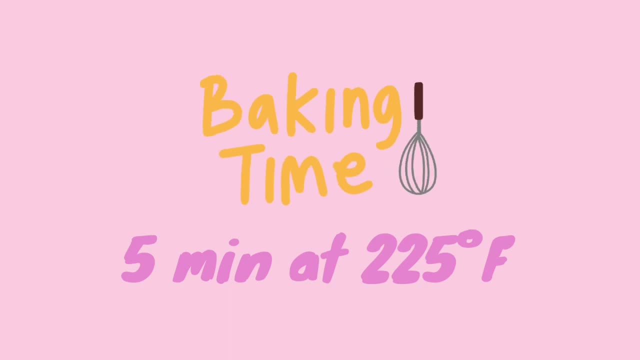 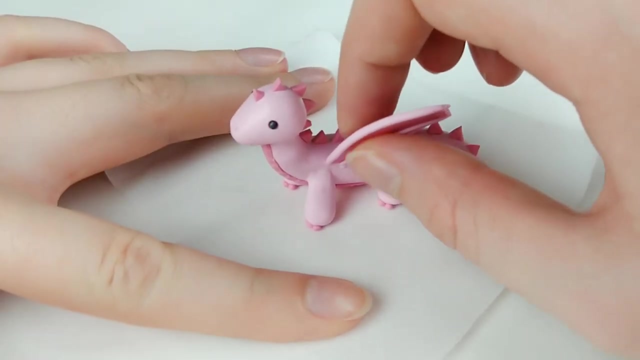 Now pre-bake these for a few minutes, and then I'll show you how they turn out. I put my dragon in the freezer, so pushing the wings into the clay wouldn't disturb the shape too much, but I left the dragon in the freezer a bit too long, so it was still a struggle to 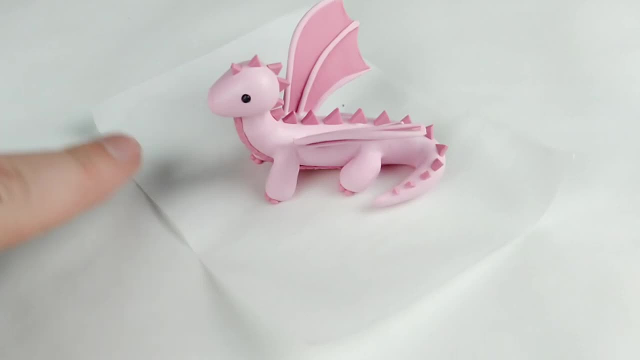 get them in. But once they're in, all that's left to do is bake our dragon a final time and we are done. I think the triangular scales are such a classic dragon look, so I'm really happy with how this one turned out. So be sure to look out for future dragon videos. 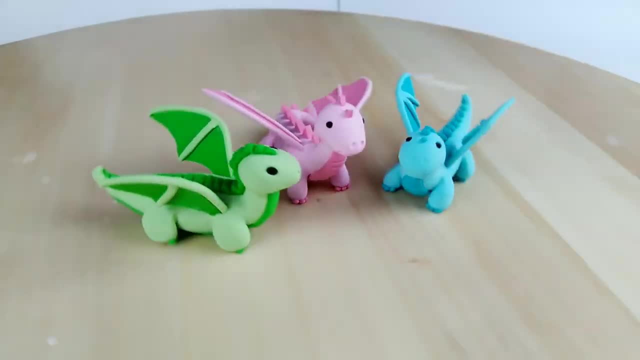 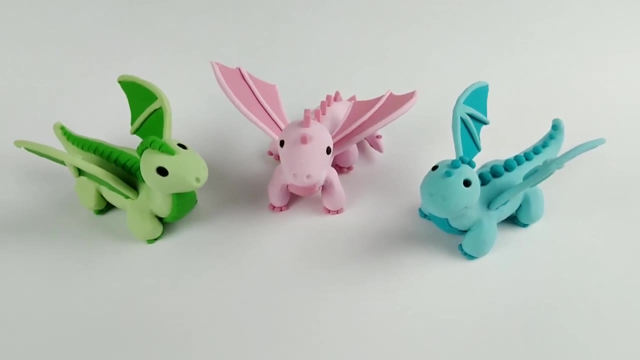 But for now, I'd love to hear which dragon was your favourite, or which combo would you have chosen for your custom dragon. But other than that, hope you have a great rest of your day and I'll see you guys later. Bye. 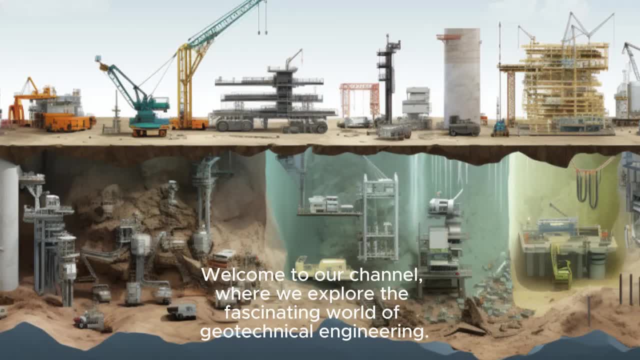 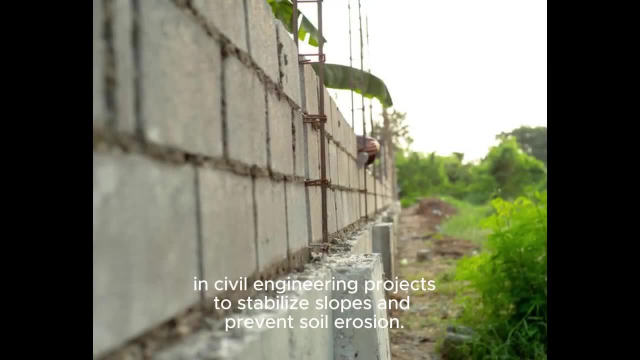 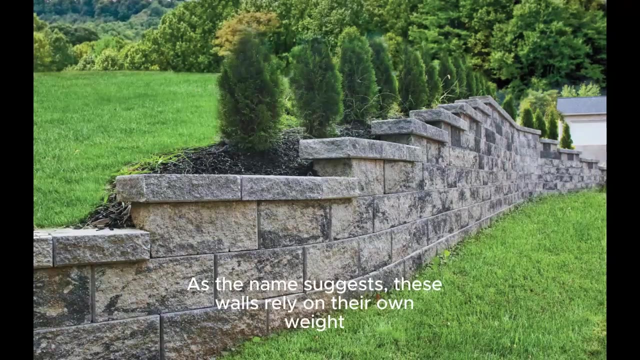 Welcome to our channel where we explore the fascinating world of geotechnical engineering. Today we'll delve into the different methods of retaining walls in civil engineering projects to stabilize slopes and prevent soil erosion. First up, we have the gravity retaining wall. As the name suggests, these walls rely on their own weight to resist the pressure of the soil. 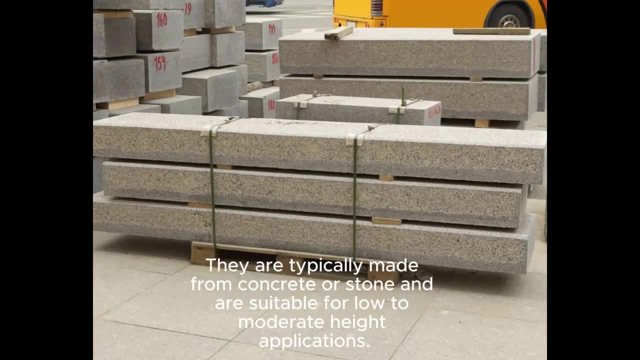 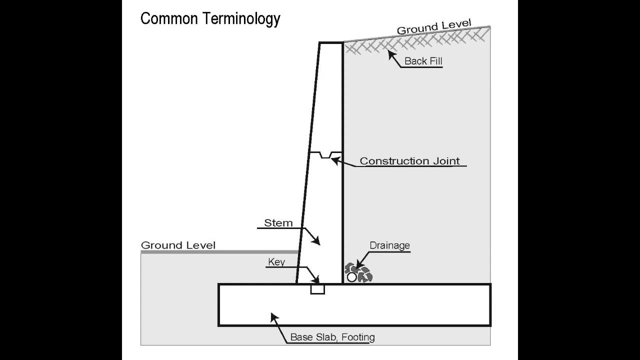 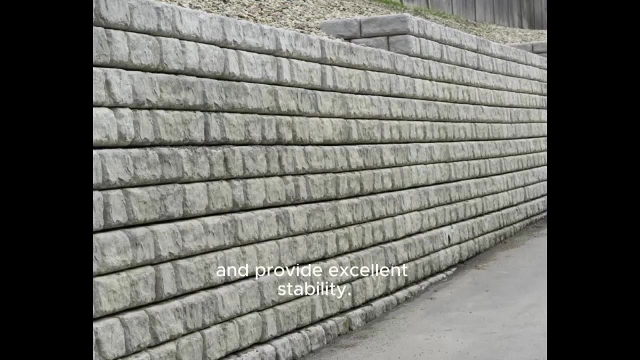 behind them. They are typically made from concrete or stone and are suitable for low to moderate height applications. Next, we have the cantilever retaining wall. These walls are designed with a reinforced concrete base and a stem that extends backwards into the retained soil. They are ideal.